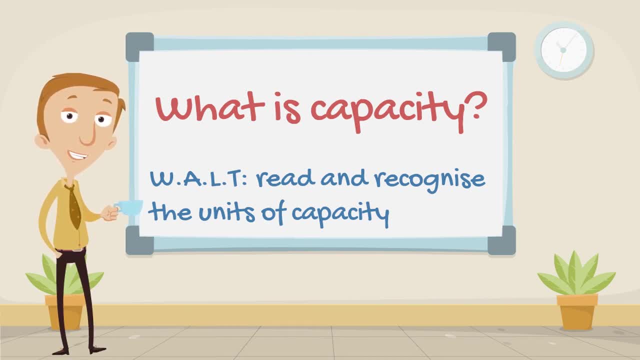 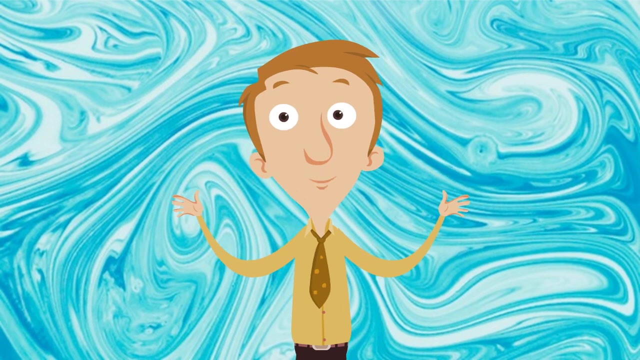 Hello and welcome back to Wrong Mar. In today's maths lesson we're taking a first look at capacity. Our goal for today is to be able to read and recognize the units of capacity. Over the last two weeks we've been looking at different units of measurement. We've looked at 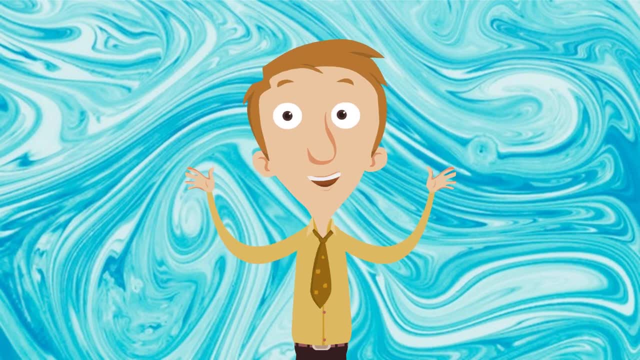 how we measure length, and we've also looked at how we measure weight. Today we've got one last type of measurement left to look at, and that is capacity. What do you think we are talking about when we say we're measuring the capacity of something? Pause the video and write down an answer. 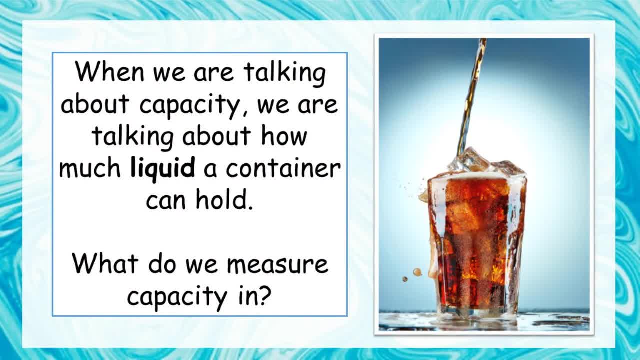 Well, when we talk about capacity, we're talking about how much liquid a container can hold inside of it, Just like this glass of coke over here. What we're talking about when we're talking about capacity is more like a scheduling signal. Just like length and weight. there are units of measurement we use for capacity. 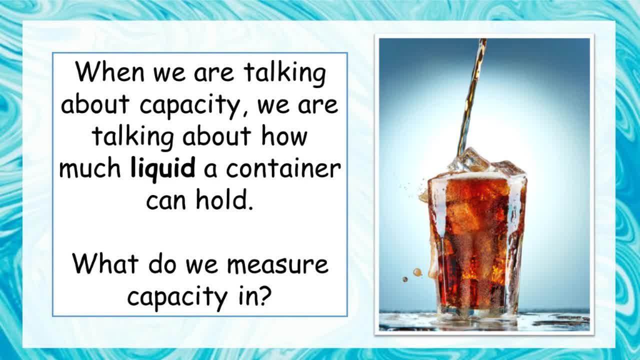 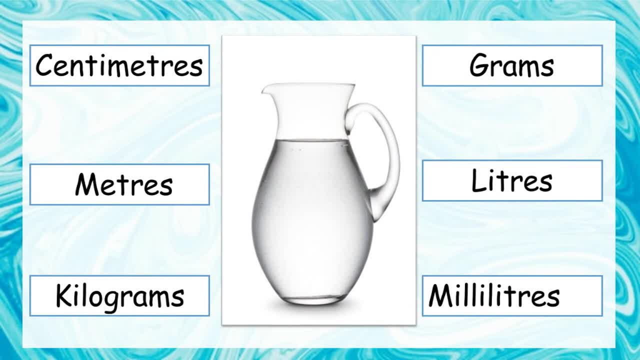 But what do we measure capacity in? How many of us can measureND? If I wanted to fill up this jug of water, which of these units of measurement would I use to measure the amount of water in it? Pause the video and see if you can figure out. 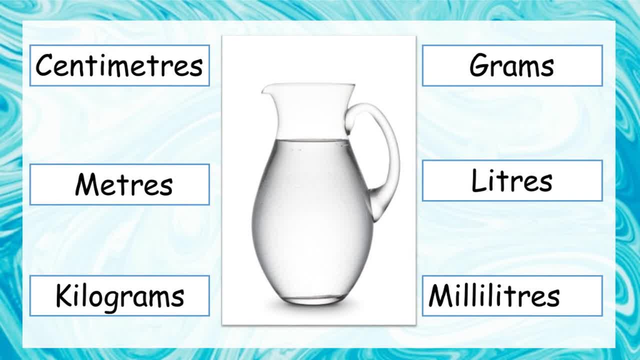 Which of these units of measurement will we measure the amount of water in? It will mean what we measure. Which are the two units of capacity? Well, did you get it right? The two units of capacity that we're looking at are milliliters and liters. 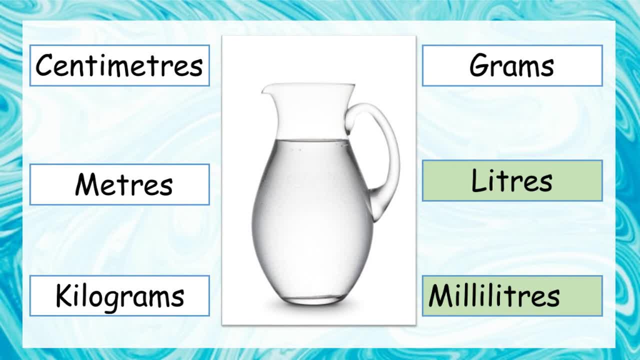 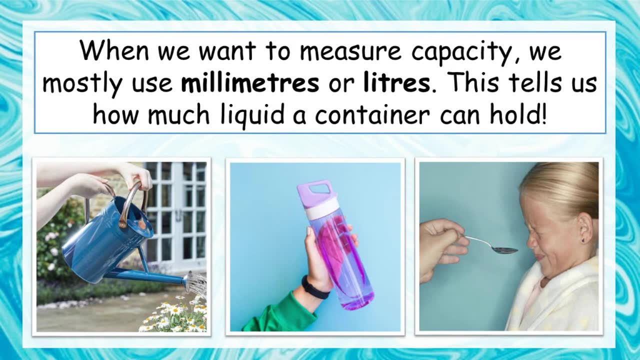 You've probably heard of these before. When we are measuring capacity, we usually measure it in liters if it's a larger item, or milliliters if it's a smaller item. This will tell us how much liquid the container can hold. 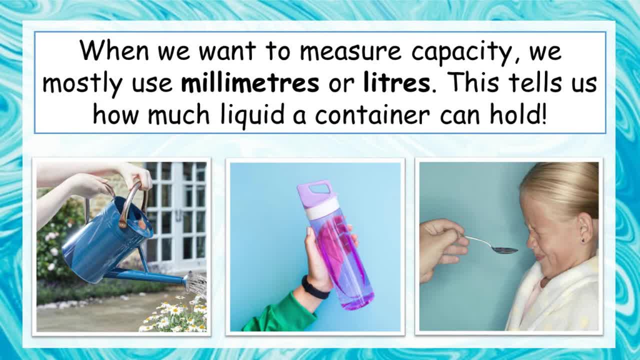 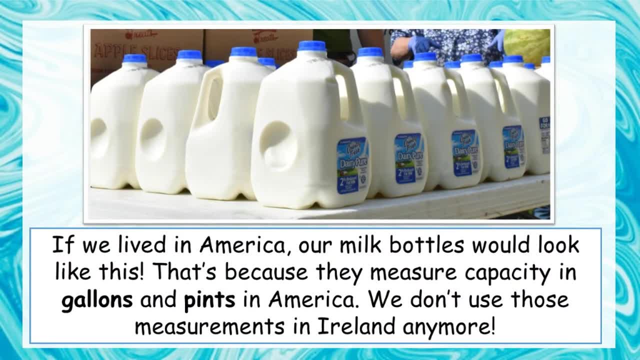 And a container can be anything. It could be a watering can, it could be a water bottle, it could even be a teaspoon. If we lived in America, our milk bottles would look like this. That's because they measure capacity in a totally different unit. 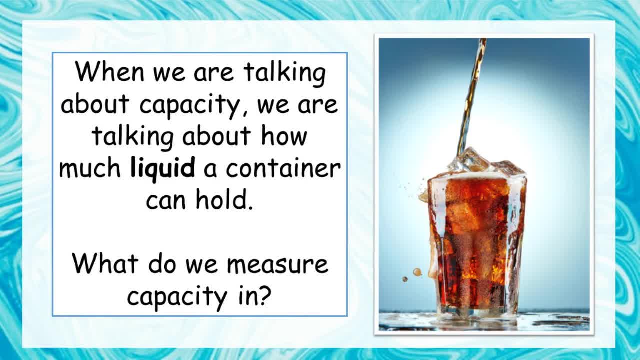 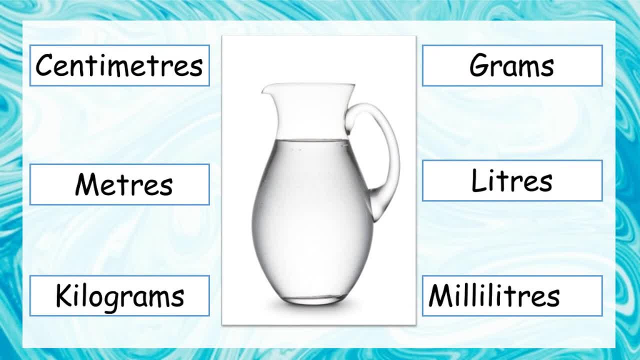 But what do we measure capacity in? If I wanted to fill up this jug of water, which of these units of measurement would I use to measure the amount of water in it? Pause the video and see if you can figure out which are the two units of capacity. Well, did you get it right? The two units of. 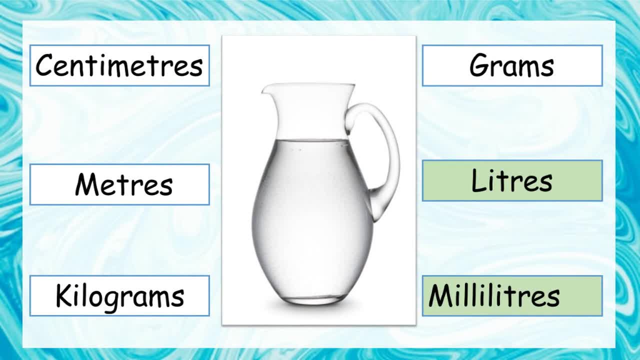 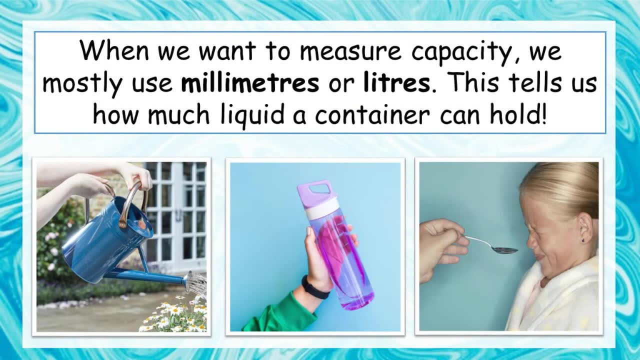 capacity that we're looking at are milliliters and liters. You've probably heard of these before. When we are measuring capacity, we usually measure it in liters if it's a larger item, or milliliters if it's a smaller item. This will tell us how much liquid the container can hold and the container can. 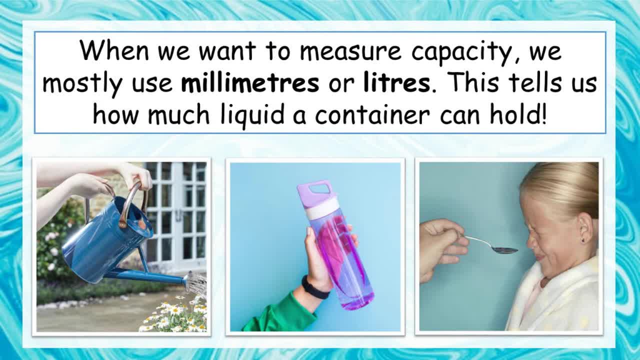 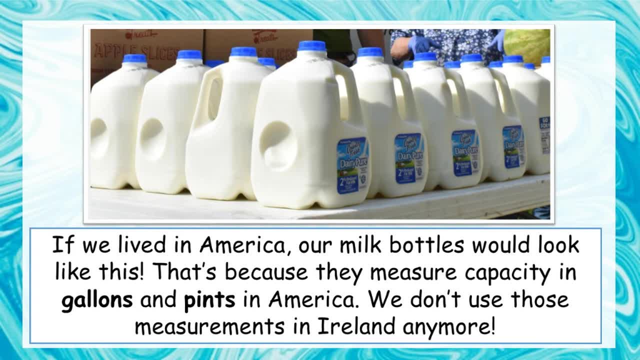 be anything. Could be a watering can, it could be a water bottle, it could even be a teaspoon. If we lived in America, our milk bottles would look like this. That's because they measure capacity in a totally different unit. They measure it. 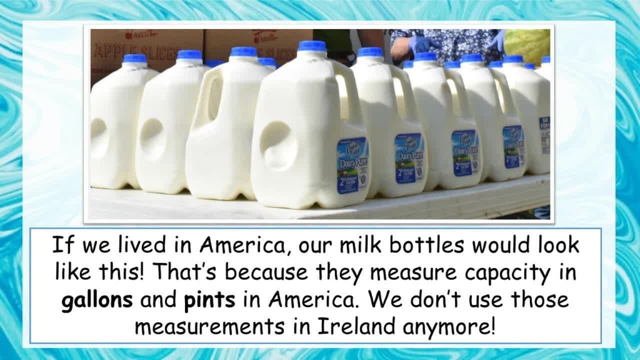 in gallons and pints. We don't use those measurements in Ireland anyway, We just do this anymore, so you really don't have to worry about them. I wonder if you could use everything you know about units of measurement that we've learnt? 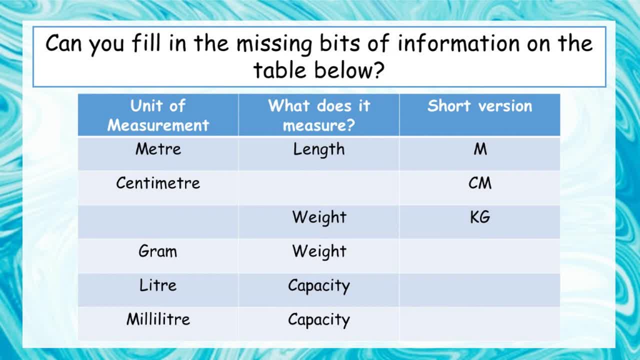 over the last few weeks and fill in the missing bits of information on the table down below. Pause the video and fill in the missing bits. Well, did you get all of those correct? So missing from the second line. centimetres are measurements of length, kilograms are: 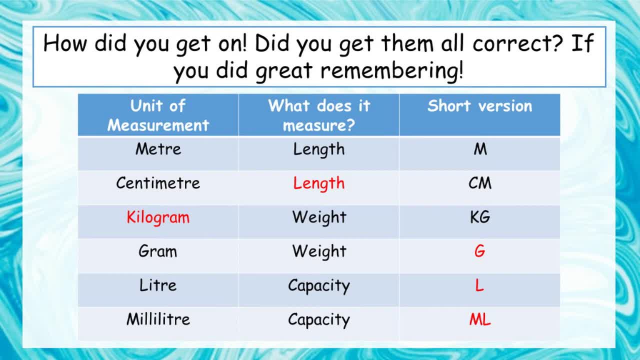 what we're talking about in the third line. g is the short version of grams, l is the short version of litres and ml is the short version of millilitres. Did you get all of them? So you probably know what question I'm going to ask next. 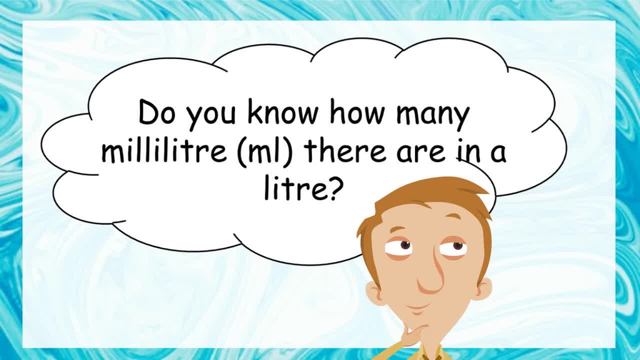 How many millilitres are there in one litre? Well, that's a good question. Think back to our other units of measurement and see if you can figure out how many there might be. Pause the video and write down an answer. Well, there are 1000 millilitres in one litre. 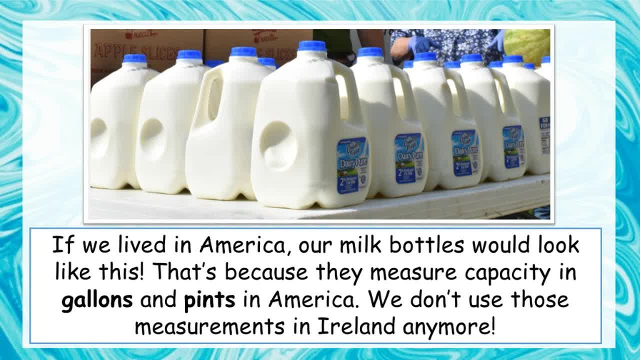 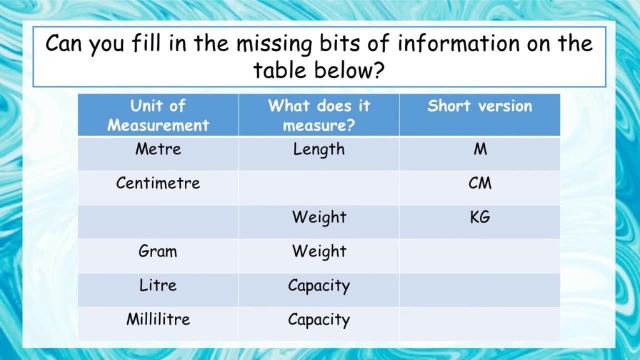 They measure it in gallons and pints. We don't use those measurements in Ireland anymore, so you really don't have to worry about them. I wonder if you could use everything you know about units of measurement that we've learned over the last few weeks. 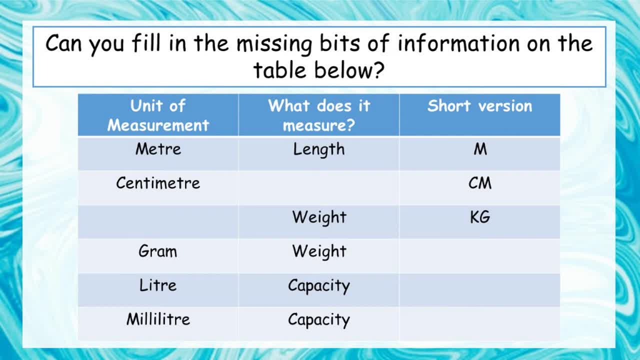 and fill in the missing bits of information on the table down below. Pause the video and fill in the missing bits. Well, did you get all of those correct? So missing bits. Moving from the second line, centimeters are measurements of length. 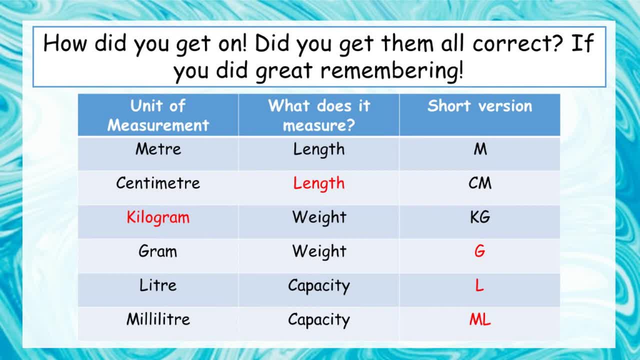 Kilograms are what we're talking about in the third line. G is the short version of grams, L is the short version of liters And ml is the short version of milliliters. Did you get all of them? So you probably know what question I'm going to ask next. 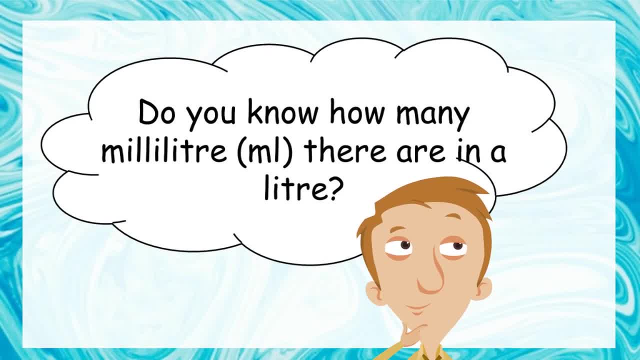 How many milliliters are there in one liter? Think back to our other units of measurement and see if you can figure out how many there might be. Pause the video and write down an answer. Well, there are 1,000 milliliters in one liter. 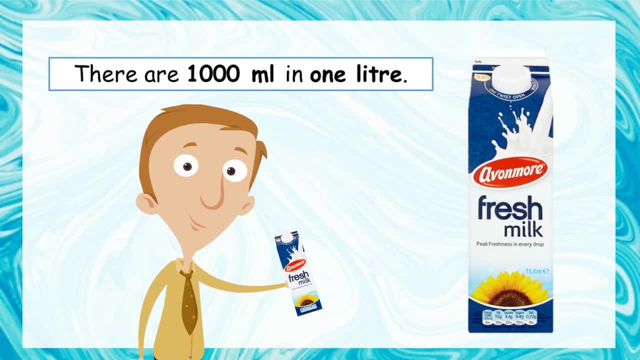 You've probably seen a liter before in your life. If you've ever seen one of these cartons of milk- the cardboard cartons, the big ones, they are usually one liter of milk. How many can be one liter? even You might even have one in your home right now. 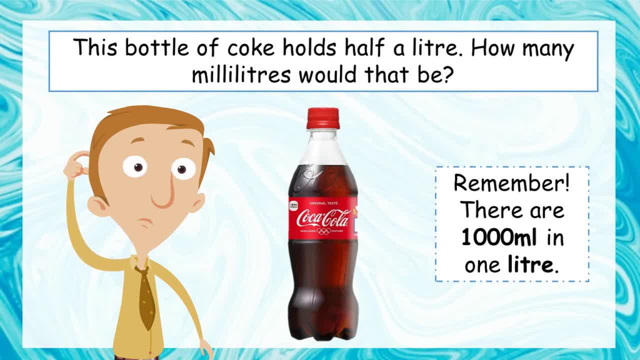 Take a look at this bottle of Coke. It holds half a liter. How many milliliters would half a liter be? Remember, there is 1,000 milliliters in 1 full liter. Pause the video and see if you can figure out how many milliliters there is in half a liter. 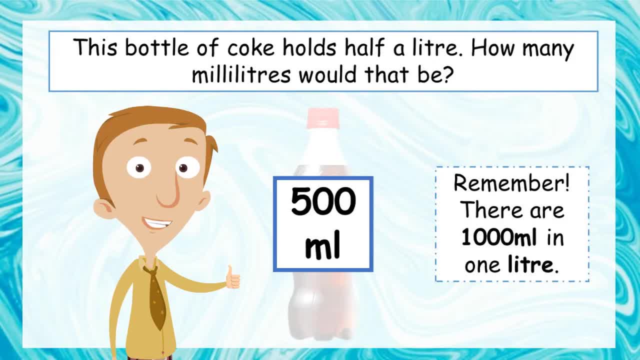 So if there is 1,000 milliliters in a liter, in a liter then there is 500 milliliters in half of a liter. Most of the small bottles of minerals that you would buy in a shop can hold 500 milliliters of liquid. Have a look. 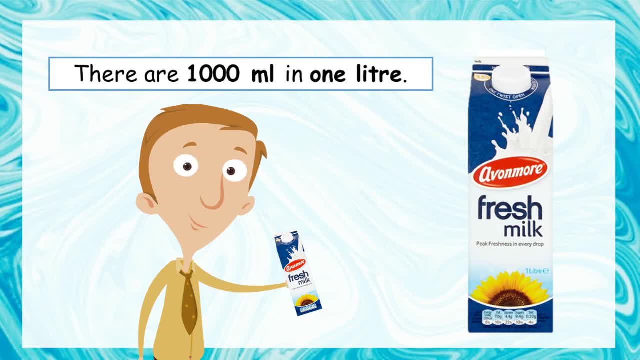 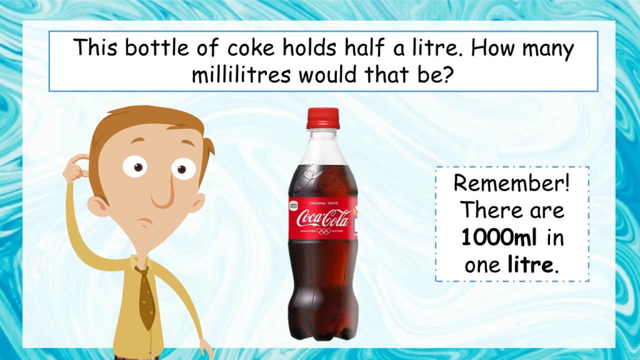 You've probably seen a litre before in your life. If you've ever seen one of these cartons of milk- the cardboard cartons, the big ones, they are usually one litre- You might even have one in your home right now. Take a look at this bottle of Coke. 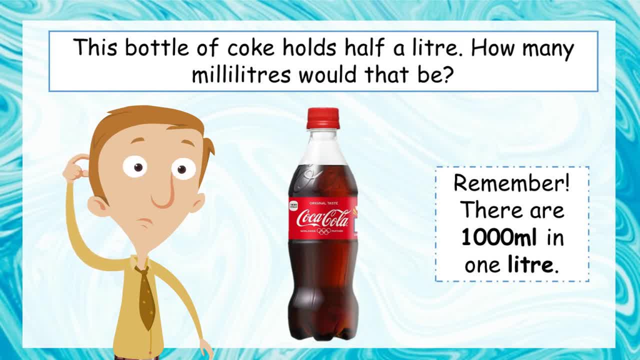 It holds half a litre. How many millilitres would half a litre be? Remember there's 1000 millilitres in one full litre. Pause the video and see if you can figure out how many millilitres there is in half a litre. 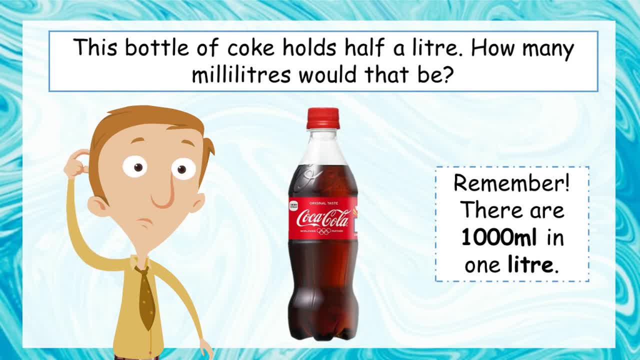 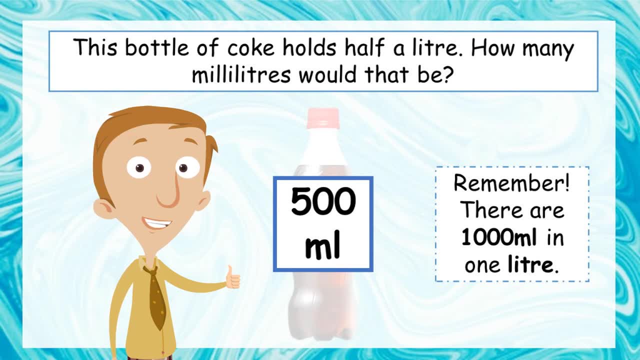 Well, if there is 1000 millilitres, you might be right, You might be wrong, You might be wrong. If there is 1000 millilitres in a litre, then there is 500 millilitres in half of a litre. 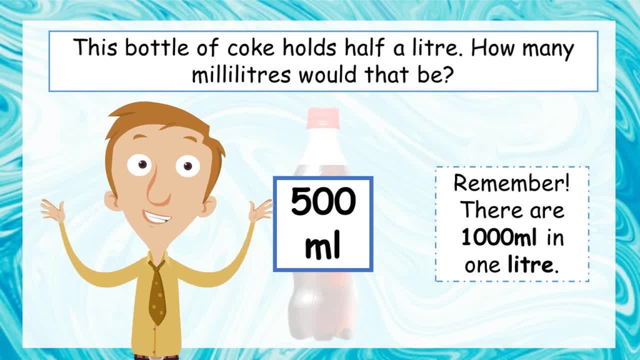 Most of the small bottles of minerals that you would buy in a shop can hold 500 millilitres of liquid. Have a look next time you're in the shop. See if you can find the measurement on the side of the bottle. Take a look at this bottle of Tropicana. 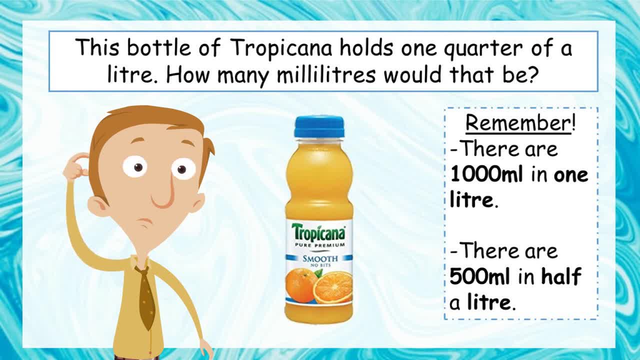 If you've ever seen one of these before, you know that they're quite small. It holds one quarter of a litre. How many millilitres would that be? Remember there are 1000 millilitres in a litre and 500 millilitres in half a litre. 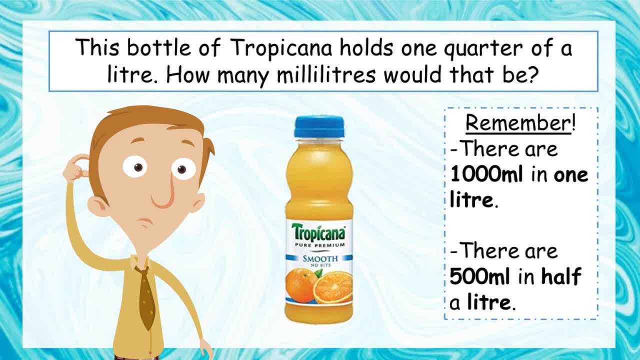 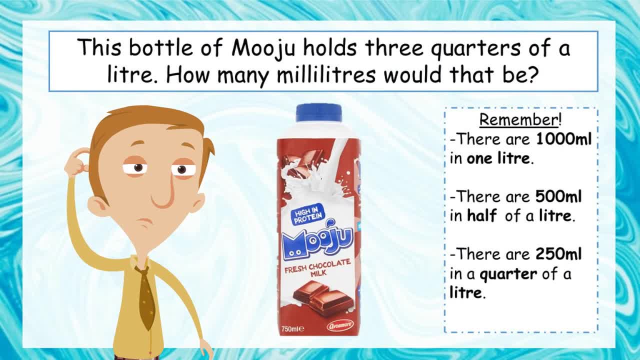 That's right. That's right, Half of a half. The final container we'll look at is this bottle of Muju. Now, I am a big fan of Muju. I think it's absolutely delicious. There's nothing I like more than a cold glass of Muju. 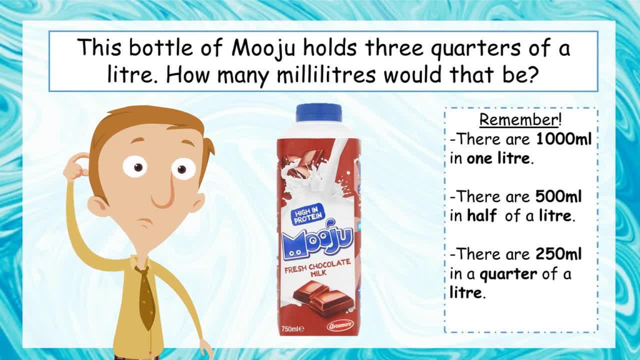 This bottle holds three quarters of a litre. How many millilitres would that be? Remember there are 250 millilitres in one quarter And 1000 millilitres in one litre. So how many millilitres would three quarters be? 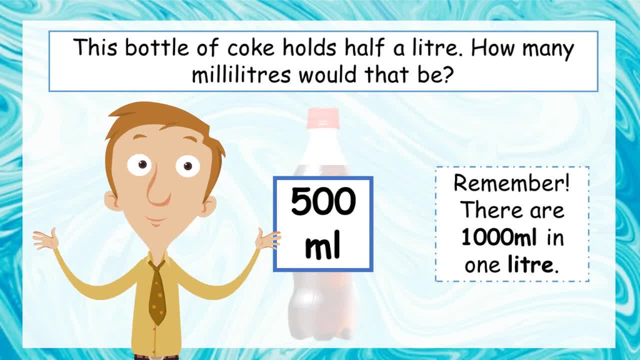 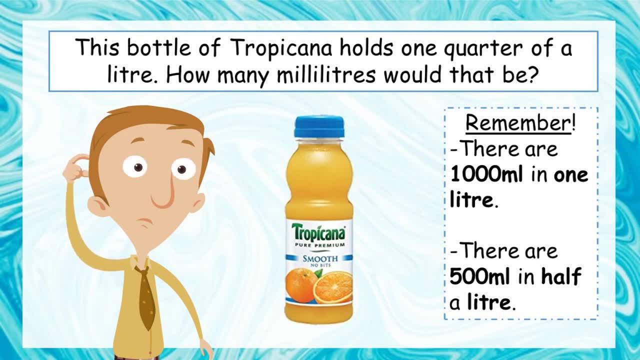 next time you're in the shop, see if you can find the measurement on the side of the bottle. Take a look at this bottle of Tropicana. If you've ever seen one of these before, you know that they're quite small. It holds one quarter of a liter. How many milliliters would 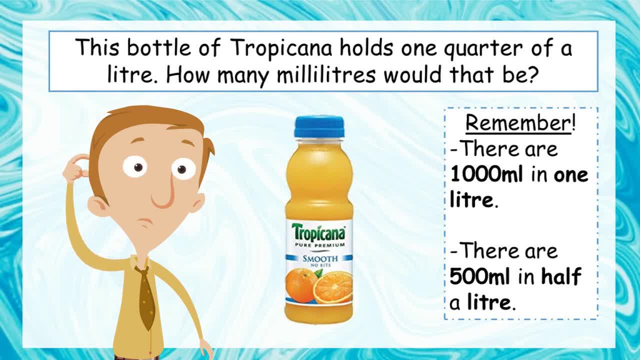 that be Remember. there are 1000 milliliters in a liter and 500 milliliters in half a liter. So how many would there be in a quarter of a liter? Pause the video and write down an answer. Well, one quarter of a liter is 250 milliliters. 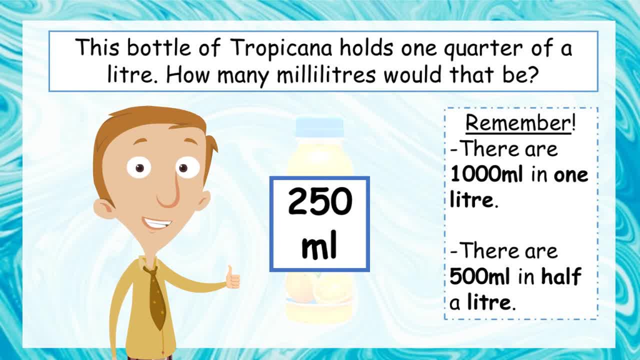 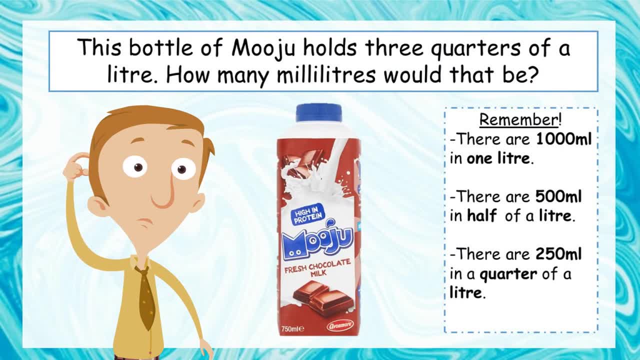 Half of a half. The final container we'll look at is this bottle of Muju. Now, I am a big fan of Muju. I think it's absolutely delicious. There's nothing I like more than a cold glass of Muju. 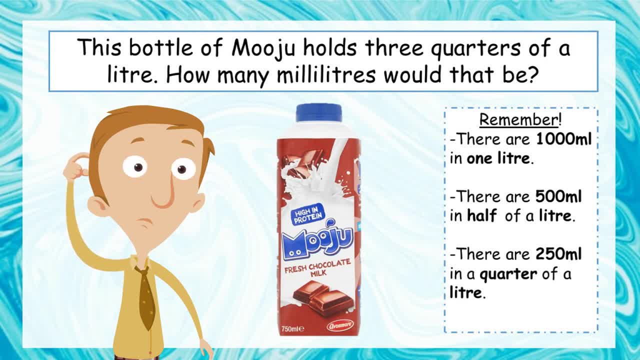 This bottle holds three quarters of a liter. How many milliliters would that be? Remember, there are 250 milliliters in a liter. Well, now that I've taken a look at another bottle like that, I'm going to look at the 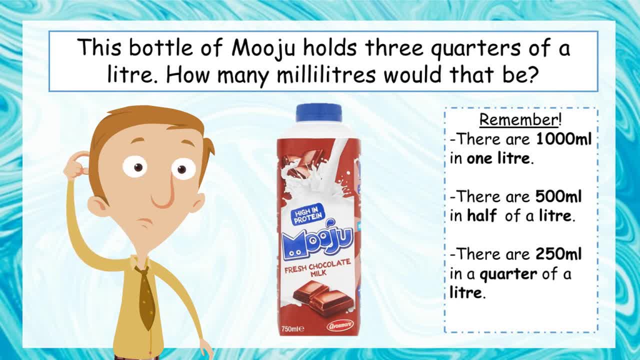 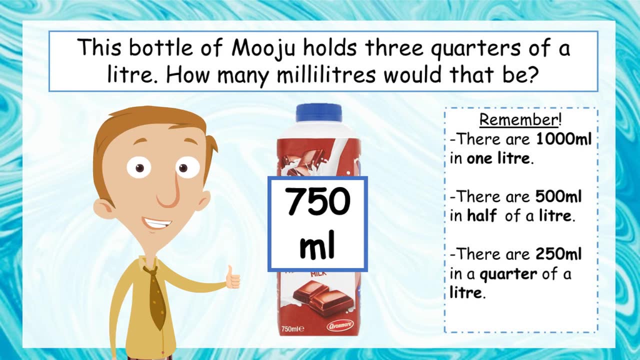 middle part: 1.3 mililiters in one quarter and 1000 milliliters in one liter. How many milliliters would that be? Pause the video and write down an answer. Well, three quarters of a liter is 750 milliliters. Did you get that? If you did, good job Well. 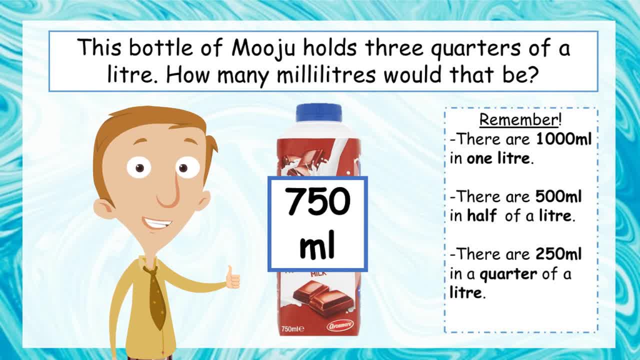 done If you didn't try to learn those little conversion facts off by heart. They'll help you understand. they'll help you a lot as we go forward. Okay, let's practice a few milliliter liter questions. I'm going to show you a picture of a container filled with. 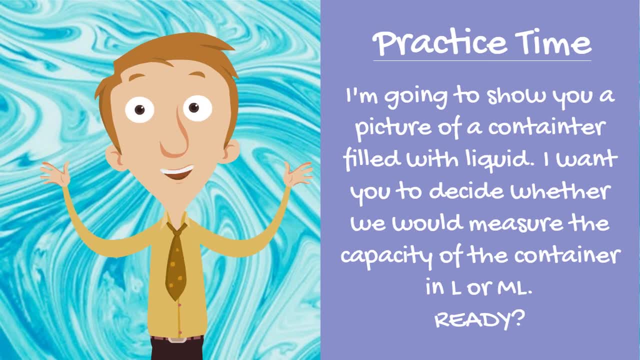 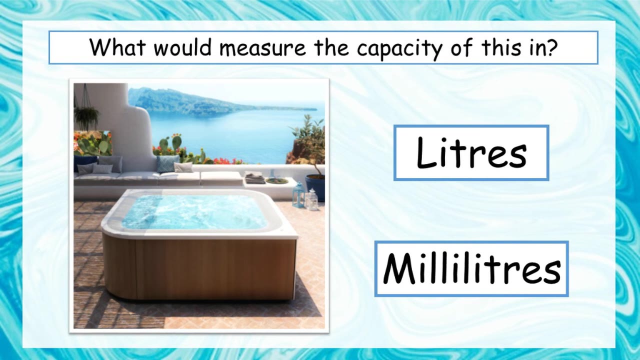 liquid. All I want you to do is to decide whether we would measure the capacity of the container in liters, or would it be better to measure it in milliliters? You ready? Okay, let's jump into our first container. I don't mind literally jumping. 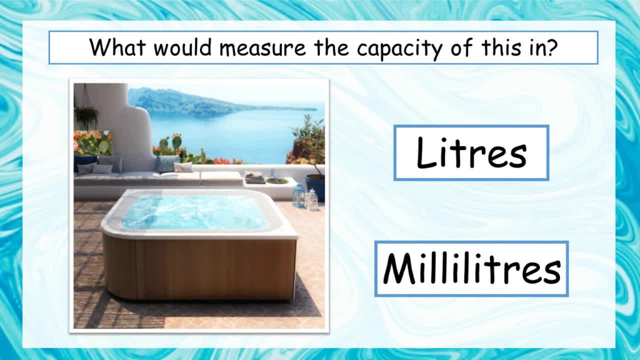 into this container? We have a lovely hot tub here, with a beautiful view, and it's filled with water. What would you measure the capacity of this hot tub in Liters or milliliters? Pause the video and write down an answer. Well, of course. 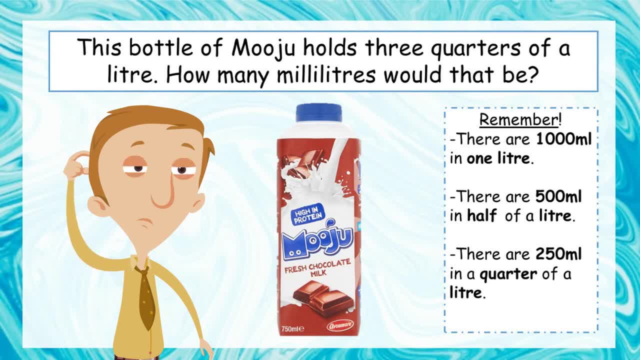 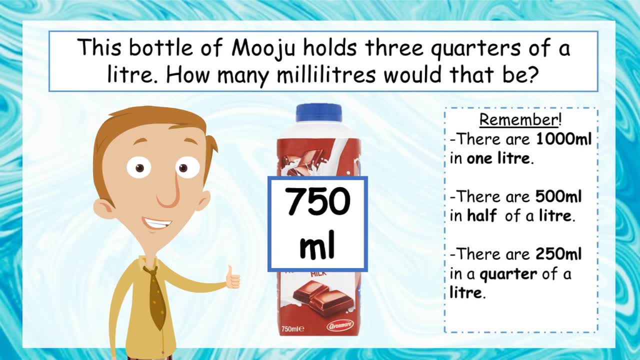 Pause the video and write down an answer. Well, three quarters of a litre is 750 millilitres. Did you get that? If you did, good job, Well done, If you didn't try to learn those little conversion facts off by heart. 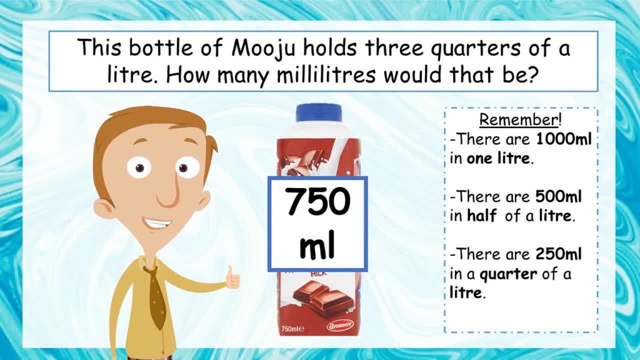 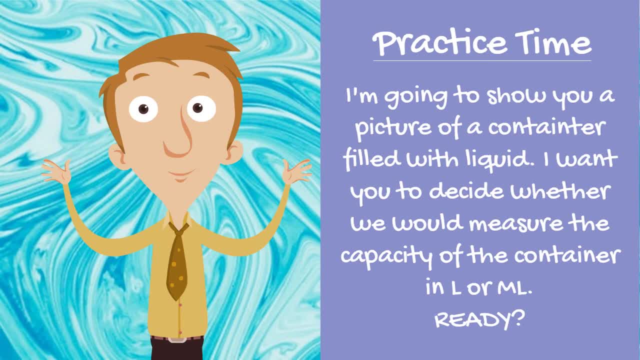 They'll help you a lot as we go forward. Okay, let's practice a few millilitre-litre questions. I'm going to show you a picture of a container filled with liquid. All I want you to do is to decide whether we would measure the capacity of the container. 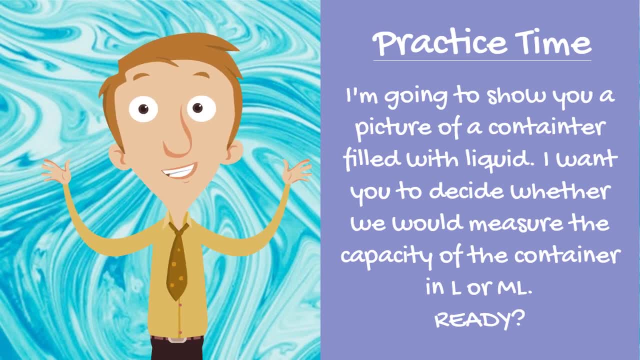 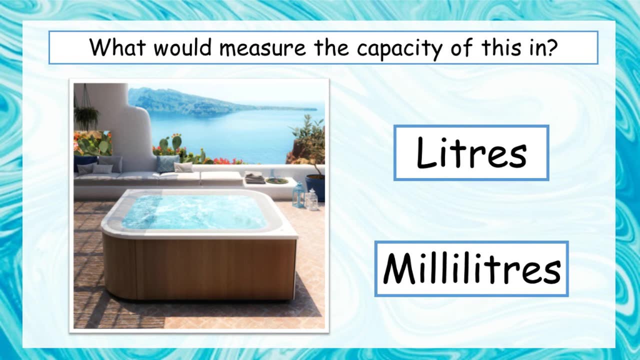 in litres, or would it be better to measure it in millilitres? You ready? Okay, let's jump into our first container. I wouldn't mind literally jumping into this container. We have a lovely hot water bottle. We have a lovely hot tub here with a beautiful view, and it's filled with water. 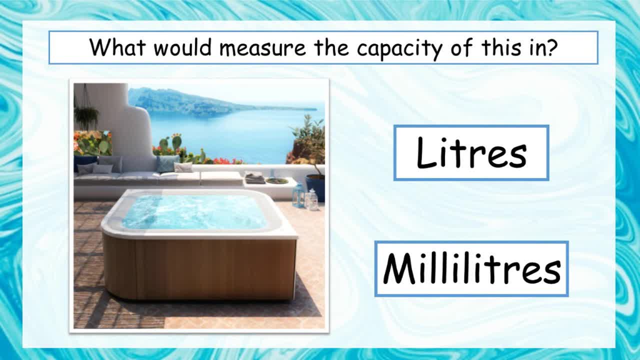 What would you measure the capacity of this hot tub? in Litres or millilitres? Pause the video and write down an answer. Well, of course, for a container this big, we would definitely measure it in litres. So give yourself a tick if you got that one right. 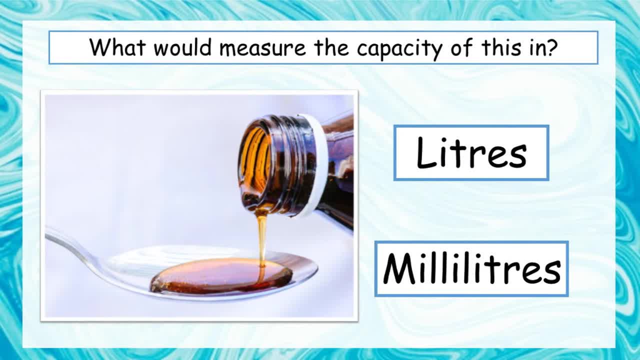 And let's go on to our second container. Okay, much smaller this time. We have a teaspoon of maple syrup, maybe for some pancakes or something. Would you measure the capacity of this spoon in litres or in millilitres? Pause the video and write down your answer. 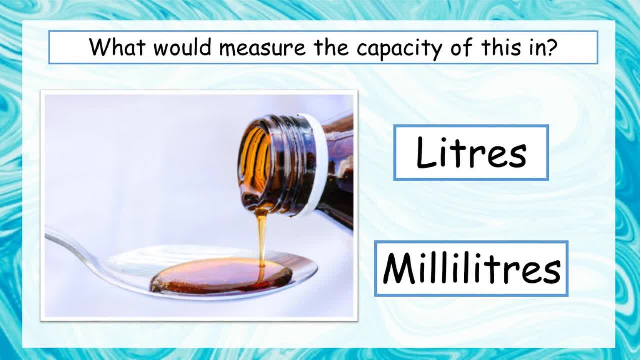 Well, of course, this container is quite small, so we would use a small unit of measurement, We would use millilitres for this one. Let's go on to our next container. Okay, So here we have a man filling up the petrol tank. 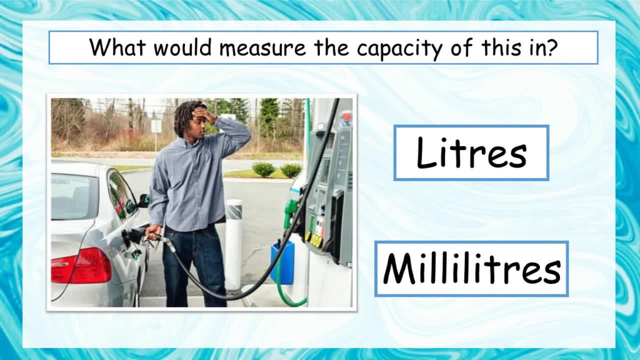 Okay, He's filling up the petrol tank on his car. Would we measure the capacity of the petrol tank in litres or in millilitres? Pause the video and write down which unit you think would be best. Well, the answer is definitely litres. 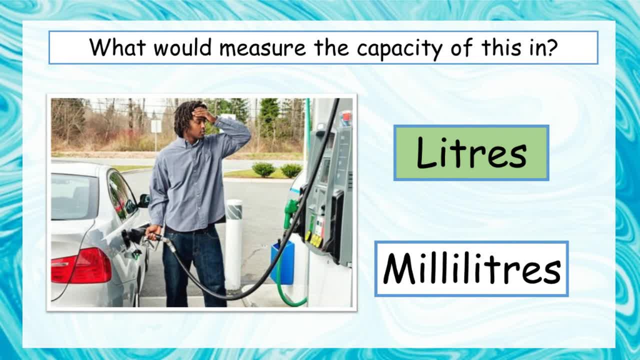 And you even see this at the petrol station pump. You should have a look out next time you're there. You can see it counts up how many litres have gone into the tank. That's how they figure out how much you have to pay. 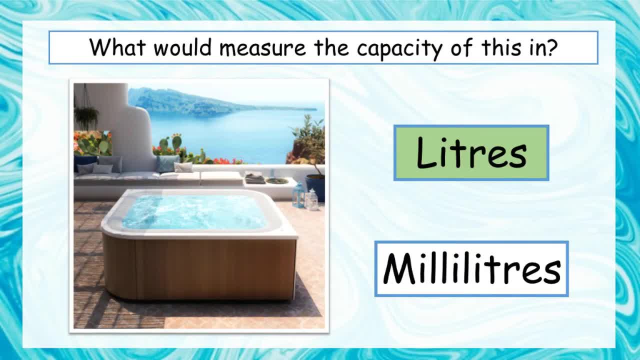 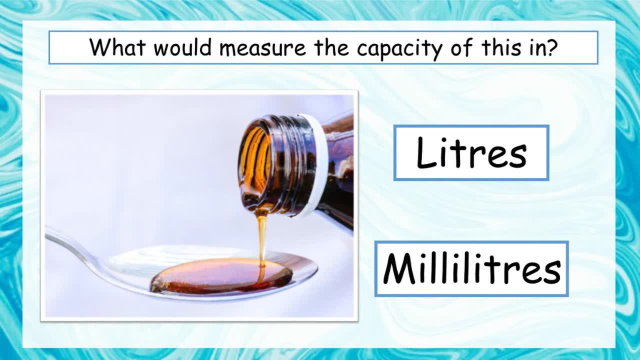 for a container this big, we would definitely measure it in liters. So give yourself a tick if you got that one right And let's go on to our second container. Okay, much smaller this time. We have a teaspoon of maple syrup, maybe for some. 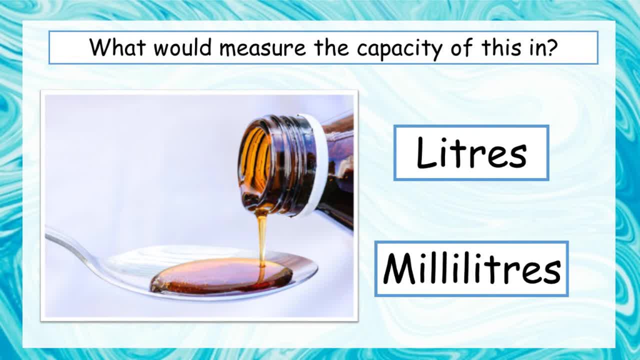 pancakes or something. Would you measure the capacity of this spoon in liters or in milliliters? Pause the video and write down your answer. Well, of course, this container is quite small, so we would use a small unit of measurement. We would use milliliters for this one. Let's go on to our next container. Okay, so here we have a. 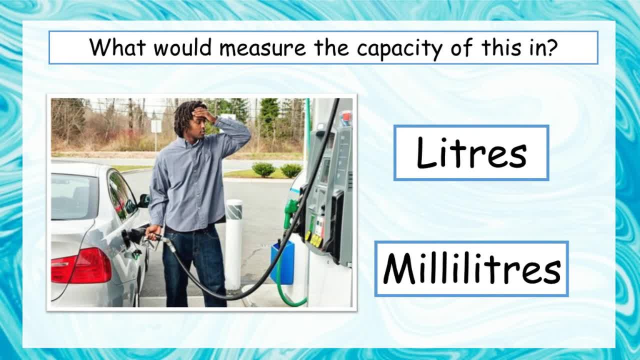 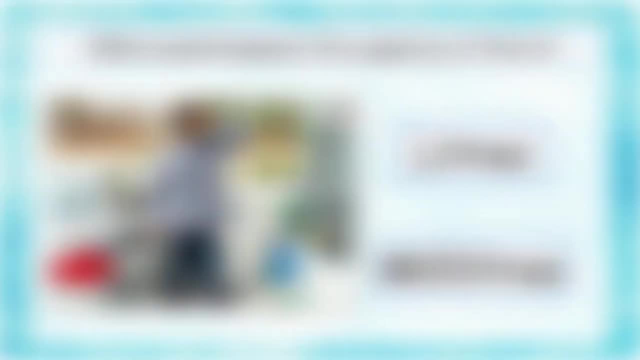 man filling up the petrol tank on his car. Would we measure the capacity of the petrol tank in liters or in milliliters? Pause the video and write down which unit you think would be best. Well, the answer is definitely liters, and you even see this at the petrol station pump. You should have a look out next time you're. 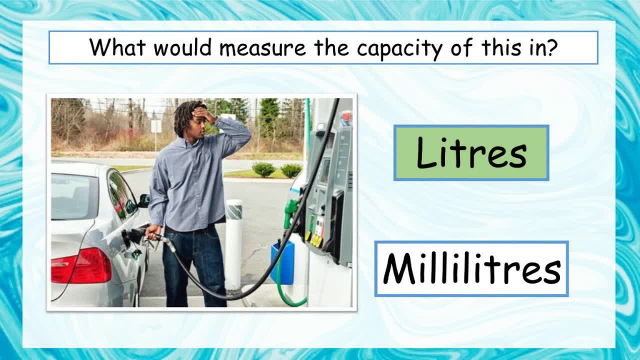 there You can see it counts up how many liters have gone into the tank. That's how they figure out how much you have to pay. You'll see the big sign at the front of the petrol station saying how much it costs per liter. Okay, next one. Ah, so we have Granny Mar is. 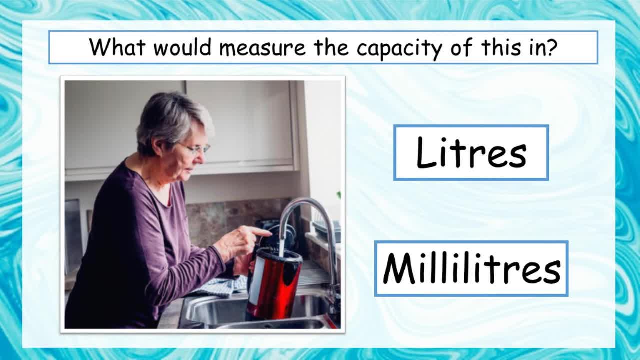 filling up the kettle to put it on for a cup of tea. Would we measure the capacity of the kettle in liters or in milliliters? Pause the video and write down your answer. Well, this is a bit of a trick question, to be honest, because if you're going to measure, 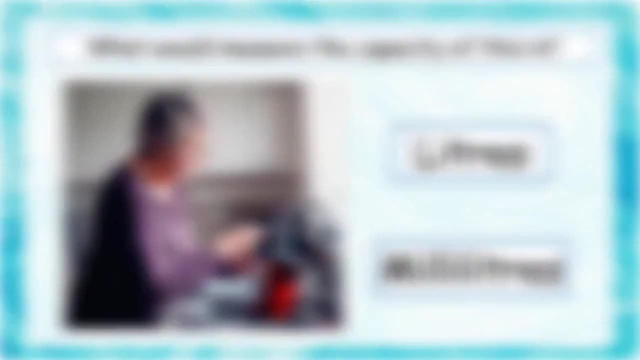 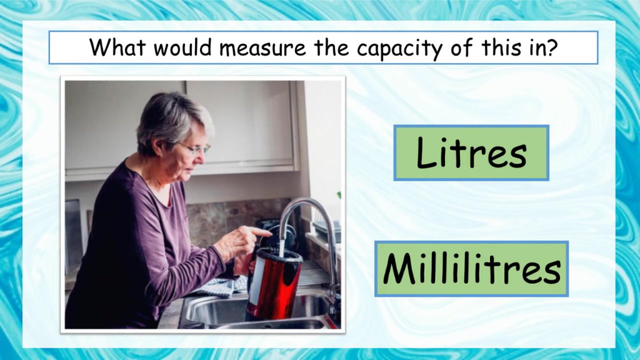 if you look at the side of your kettle, it probably has both people and liters measured on the side. I know my kettle here certainly does. It goes up in liters, but it also has marks for milliliters, so we'll go for both. So let's go to our final container. save the best till. 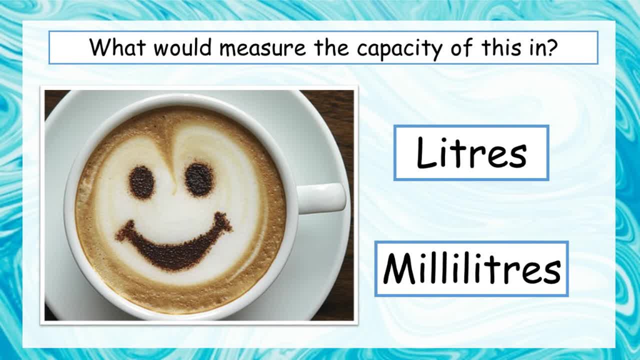 last Have a look at this cup of coffee filled with vestigious warm happiness. what would we measure of this coffee cup in? Do you think it would be liters or milliliters? Pause the video and write down an answer. Well, we would definitely measure this in milliliters. I would not recommend anybody. 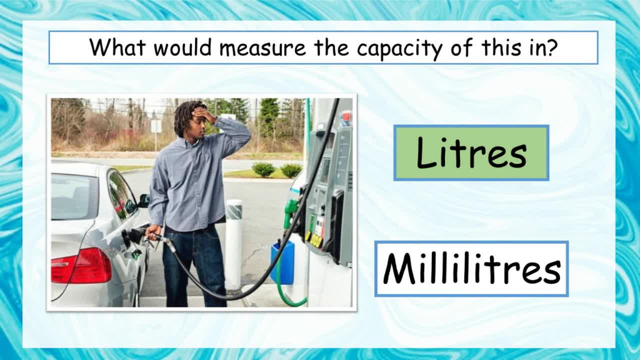 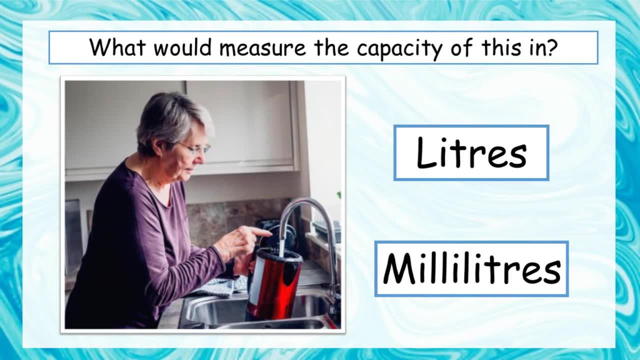 you'll see the big sign at the front of the petrol station saying how much it costs per litre. Okay, next one. Ah, so we have. Granny Mar is filling up the kettle to put it on for a cup of tea. Would we measure the capacity of the kettle in litres or in millilitres? 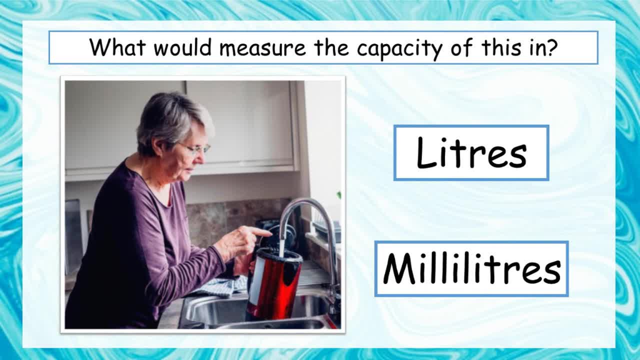 Pause the video and write down your answer. Well, this is a bit of a trick question, to be honest, because if you look at the side of your kettle, it probably has both millilitres and litres measured on the side. I know my kettle here certainly does. 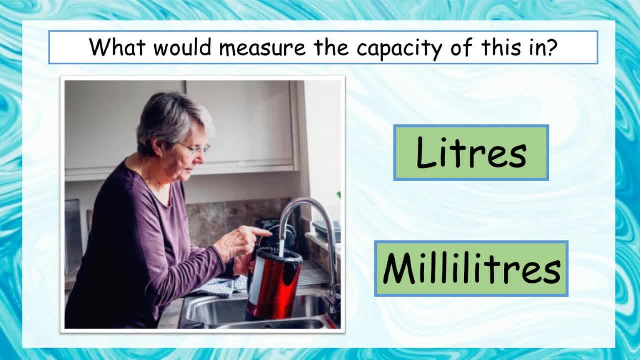 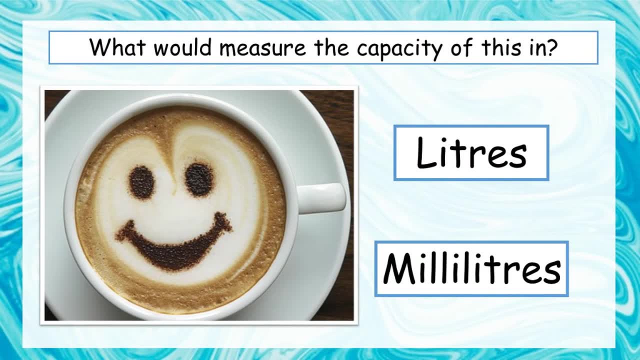 It goes up in litres, but it also has marks for millilitres, So we'll go for both. Let's go to our final container, the very last one. Save the best till last. Have a look at this cup of coffee filled with delicious, warm happiness. 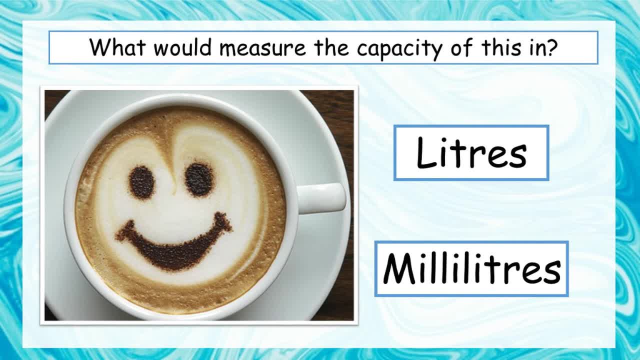 What would we measure? We would measure the capacity of this coffee cup in. Do you think it would be litres or millilitres? Pause the video and write down an answer. Well, we would definitely measure this in millilitres. I would not recommend anybody to drink litres and litres of coffee. 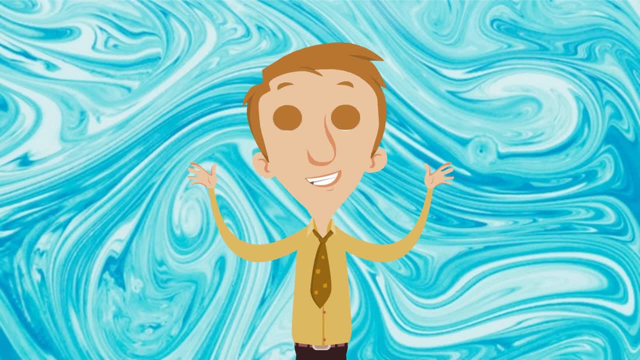 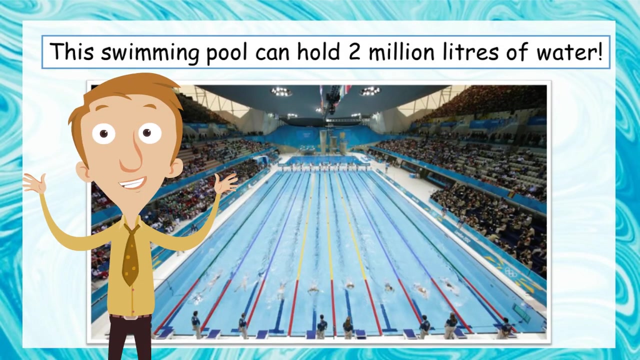 Would not be good for your heart. I don't think. How did you get on with those units of measurement questions? Did you get them all right? Let me leave you with one challenge question. This is going to get big. Here is an Olympic-sized swimming pool. 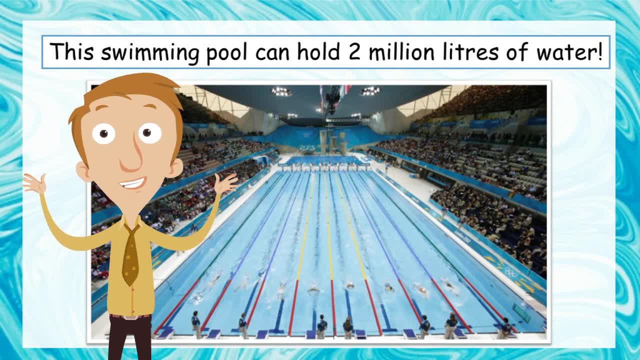 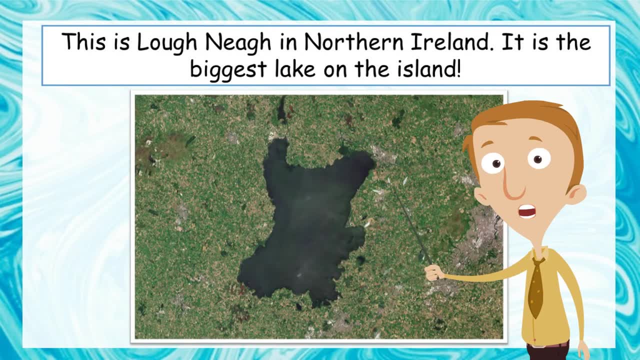 Believe it or not, this pool can hold two million litres of water. That is a huge amount of water, And here we have Loch Neagh in Northern Ireland. It's the biggest lake on the island. Here's my challenge question for you. 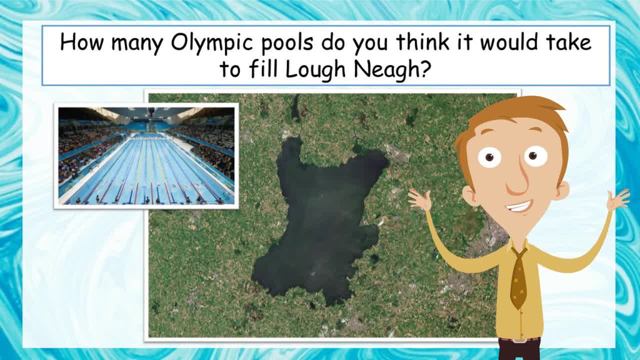 How many Olympic-sized swimming pools do you think we would need to fill up Loch Neagh with water? You can let me know what you think and I'll give a prize to anybody who can manage to get the estimate exactly right. 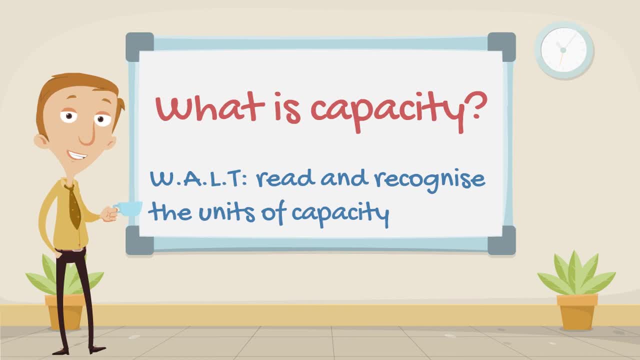 So our wall for today's lesson was to read and recognise the units of capacity, Litres and millilitres. When you're ready, you can try the practice activities down below. That's all we have time for today, Until next time.